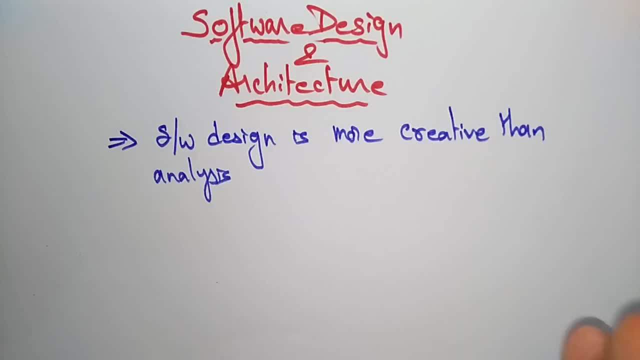 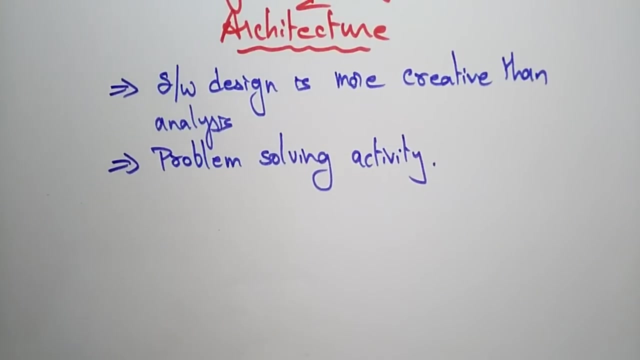 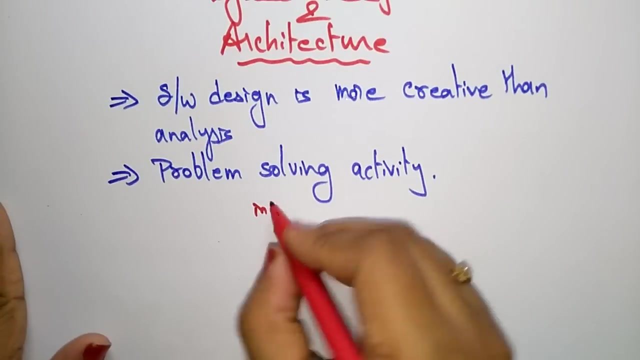 So seeing a pictorial representation is more creative, More creative than analysis. So software design is more creative than analysis. So it is also helpful for problem solving activities. It is a problem solving activity. Software designing is a problem solving activity. Okay, So actually, if you take any initial requirements, the starting, how we are going to design a software, 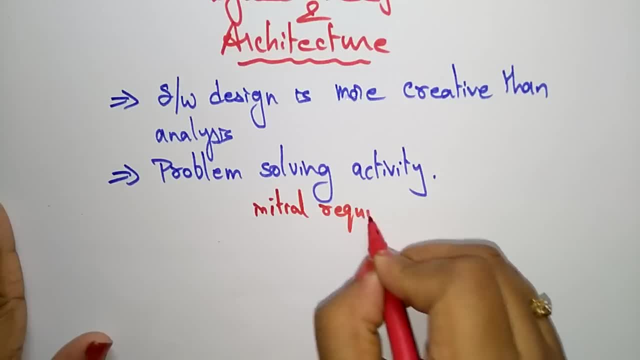 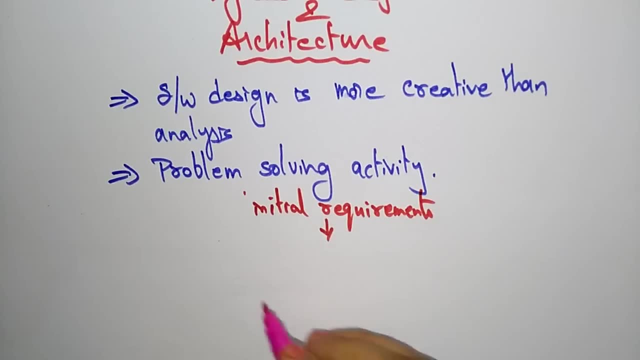 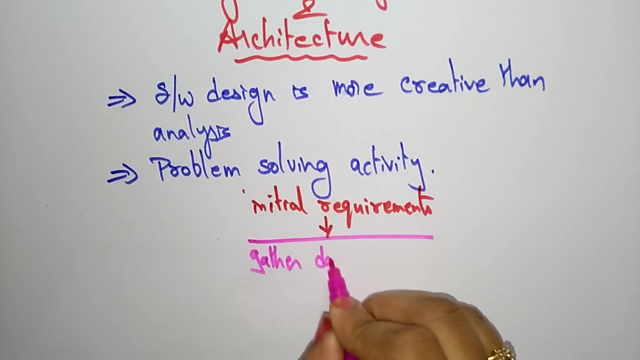 First we are taking the initial requirements, Any initial requirements from the user. Okay, So from initial requirements, first, gather data on user requirements. We have to gather the data on user requirements. So, based on the user requirements, we are gathering the data. 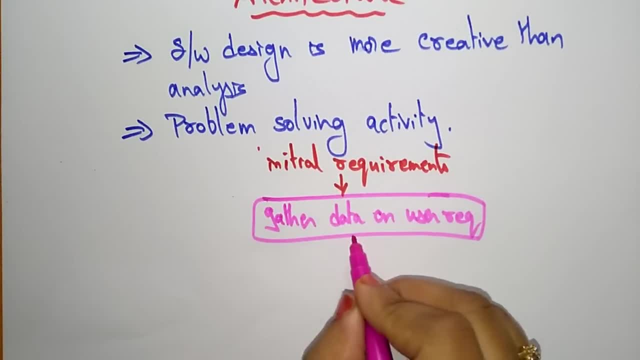 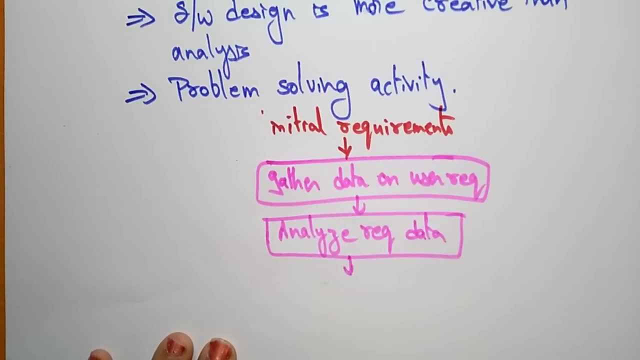 After that we are analyzing the requirements data. Let me show you Analyze requirement data. So whatever we are gathered that we have to be analyzed. So after analyzing then the conceive of high level design, We have to construct the high level design. 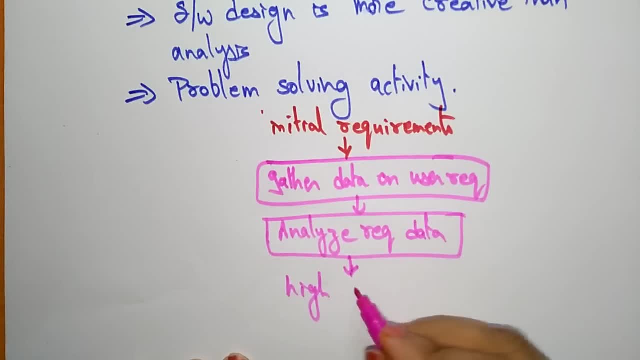 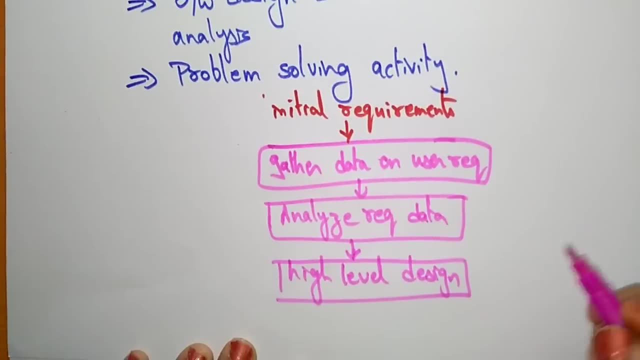 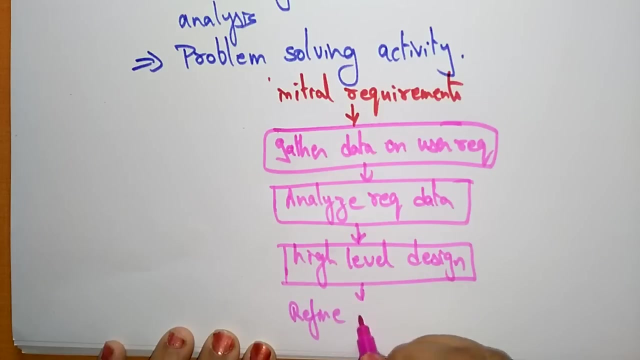 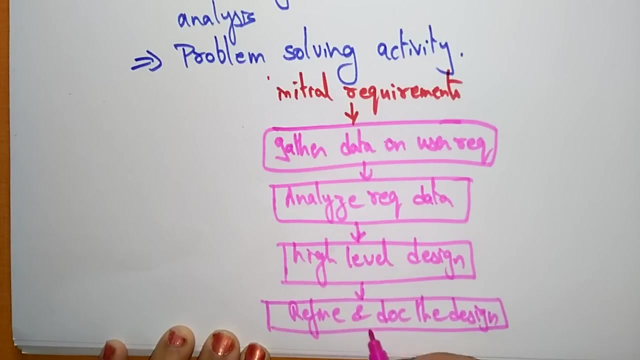 Whatever, we analyze the requirements, data that we have to be represent in the high level design. Okay, high level design is also done. Finally, we have to refine and document the design. Refine and document the design. So, whatever the pictorial representations diagrams we have given, that should be documented. 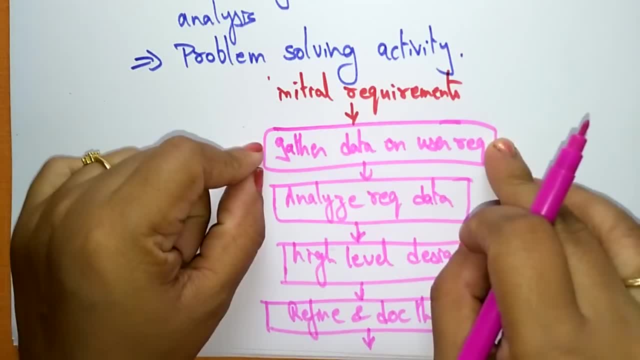 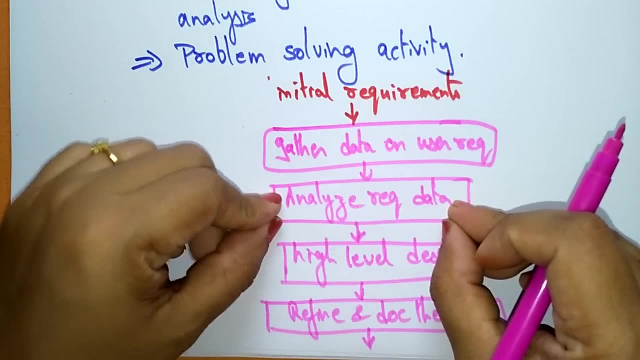 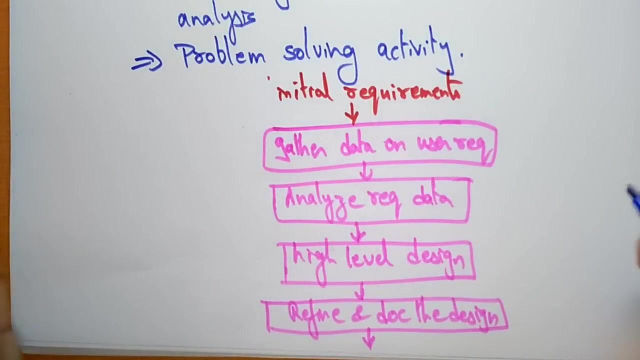 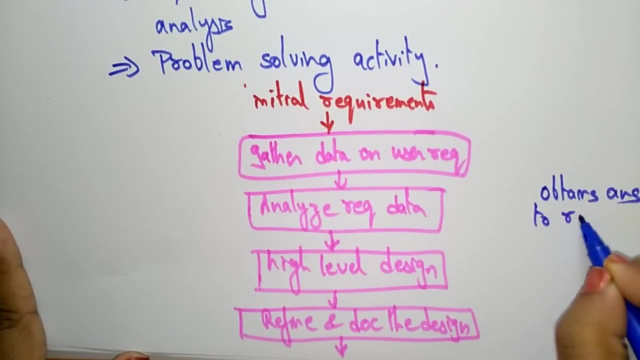 So initial requirements are taken that gather the data on user requirements and analyze the requirements data. After analyzing the requirement data, we have to design that information. Then that should be documented, Okay, and here, while doing this, it obtains answers to required requirement questions. requirement questions. 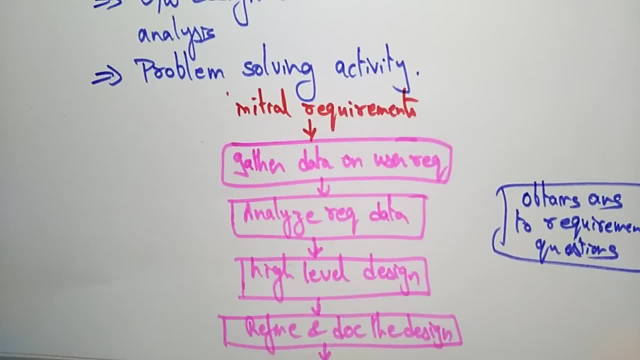 So with the help of this refine and documentation- isn't everything- we will get the answers to our questions. So how we are going to implement the project and how, What, What kind of coding we are using. Everything will be for high level designs and the refine and documentation document- the designs- we will obtain the answers to the requirement questions. 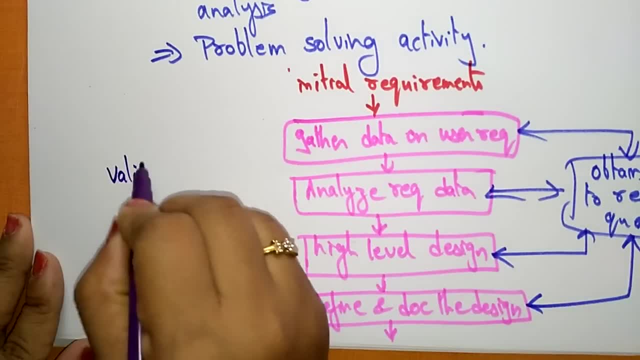 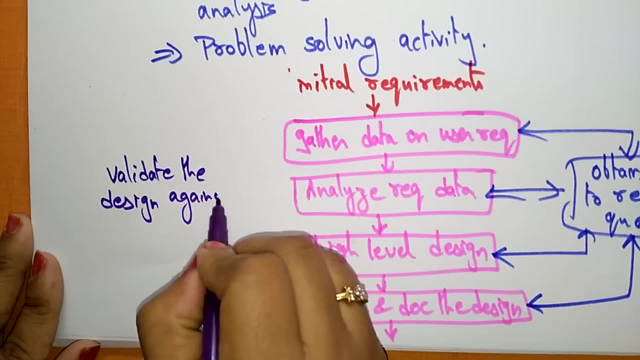 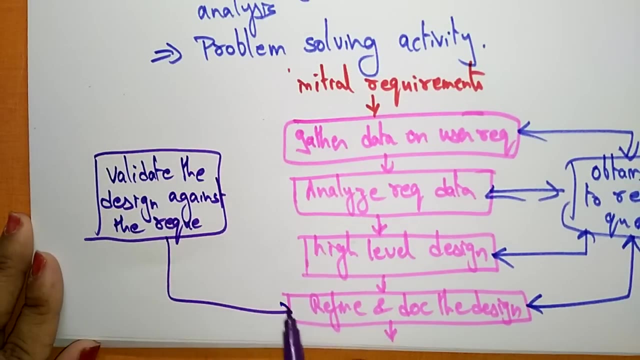 So, in the same way, it is also helpful for validate the design, validate the design again as the requirements, again as the. Every time we have to be validate the design against the requirements, every, each steps, we have to validate the design again as the requirements, again as the requirements again. 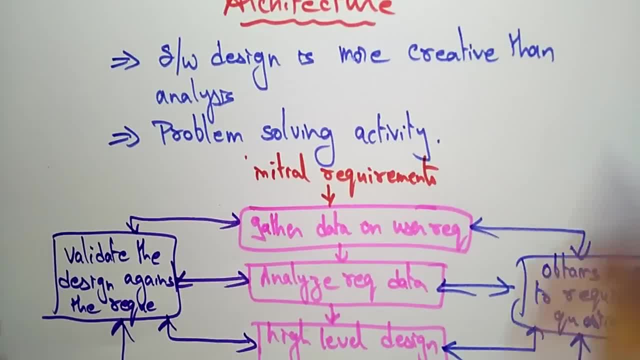 So everyone arbeitet in a way: processes the research programs, then we'll tried to draw the high level designs on thatанalyze the information, then try to draw the high level design on that requirements and refine and document the designs again as the requirements, again as the requirements. 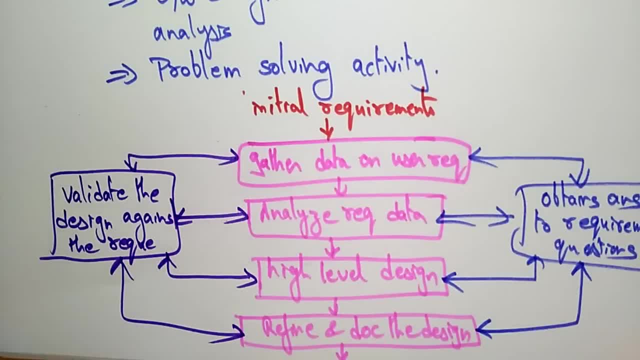 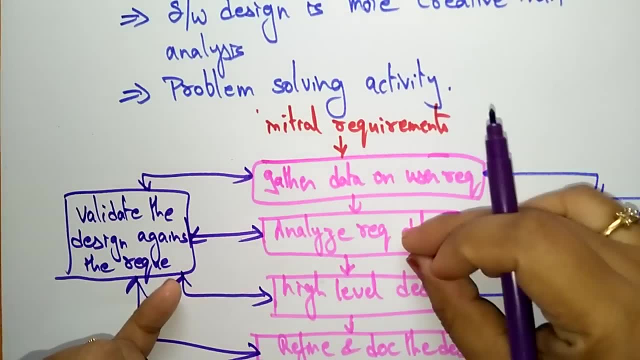 Okay, That is, you have to inform us exactly about the requirements of the project meeting center and come back once we have to do the neatly. that's the ideal structure in our stage to fill in the loyaltyitta, validate the design against the requirements and we will obtain the answers for the requirement. 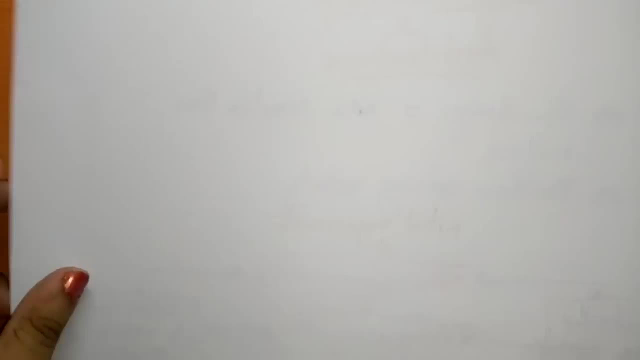 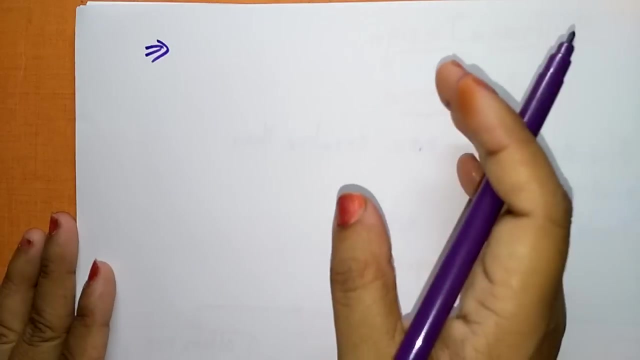 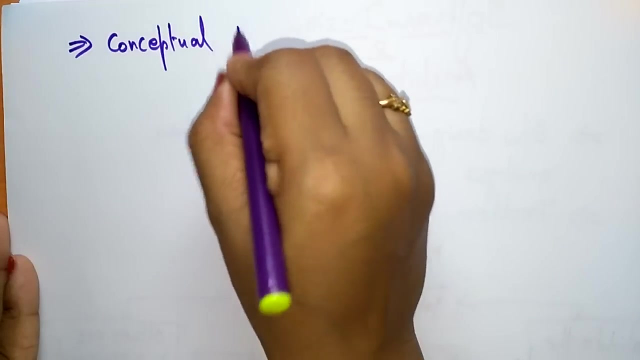 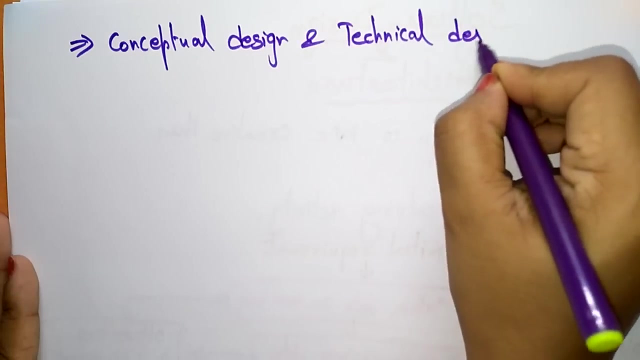 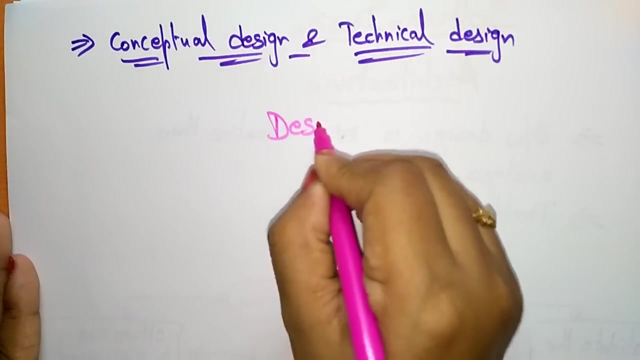 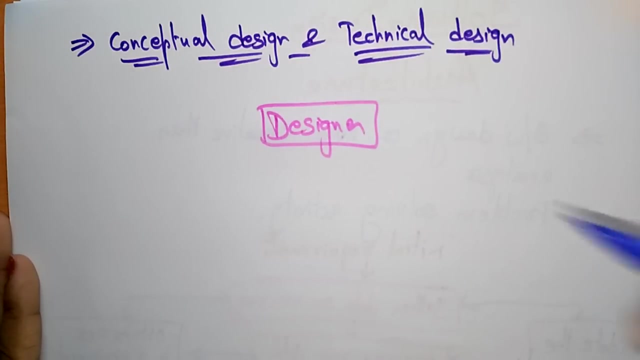 questions also. okay, now let us see: uh, there is a two parts of design process. actually, a software design is a two-part design process. one is the conceptual design: conceptual design and technical design. if you take any designer. if you take any designer means the software designers. the software designers, uh is in the form of: they can implement the. 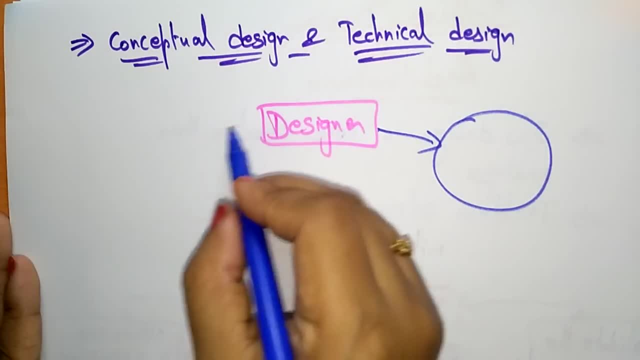 the technical design and the conceptual design. so, if it, uh, let us think, uh think about what is the, the concept of design? uh, we need to understand it. ah, if it is the concept of design, then what is the new concept of design for people in the future? is, it is the concept of design. 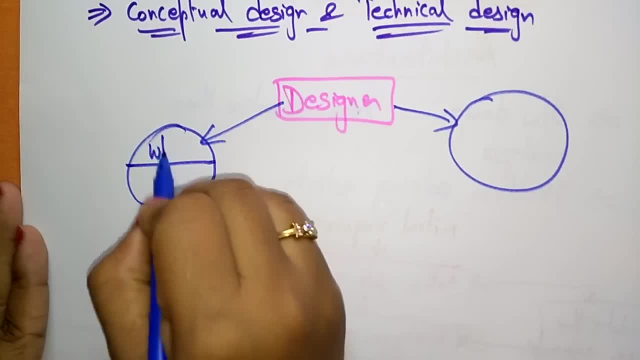 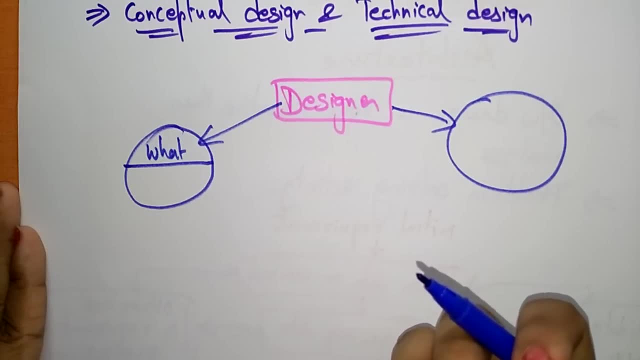 if it is anulatorsist, um, you know, we do not always that kind of uh concept is a conceptual design. so the conceptual design main things about what, what the design i means, what type of designs they are going to be implement, how the structure is going to be developed. 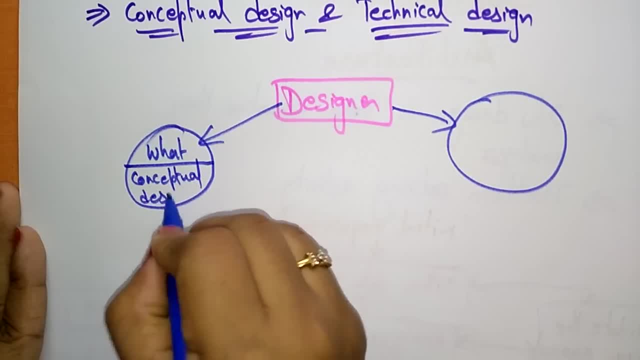 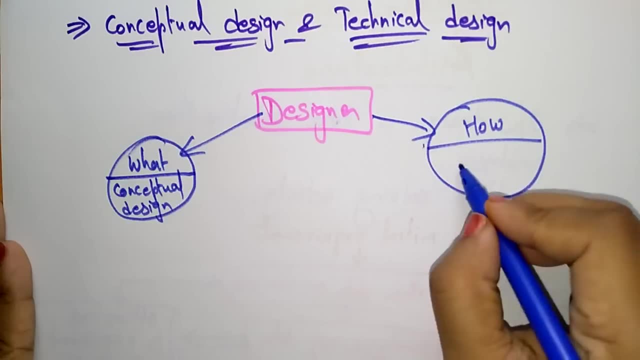 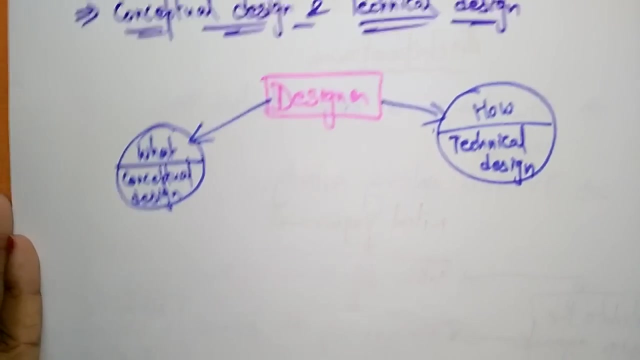 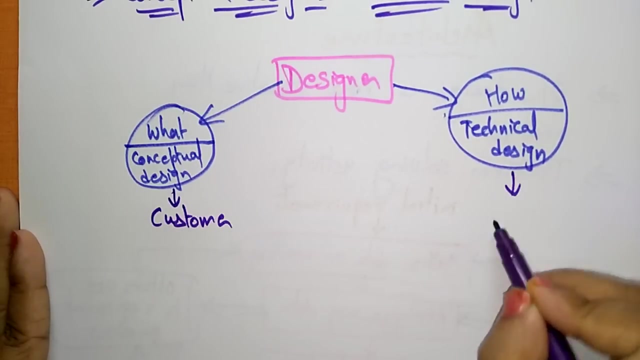 so this is, let me write first, this is a conceptual design, and here this designer: think about how. which designer, the technical designer, will thinks about always how how the project is implemented. okay, so here, uh, conceptual designer is nothing but a customer and technical designer. we call it as a system developer, system builder or system. 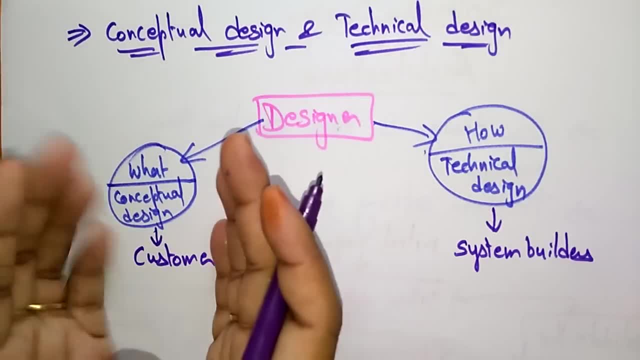 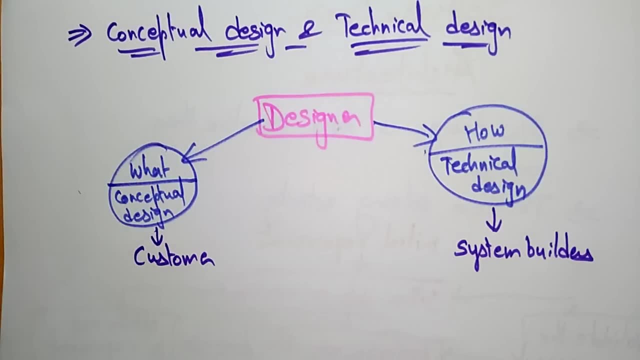 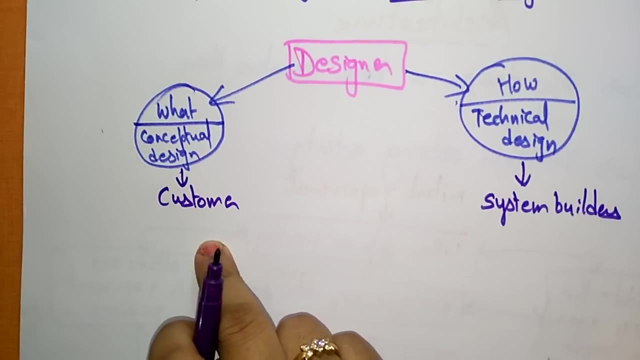 developer, any person so a conceptual means customer, technical designer is system builders, conceptual designer, what they think. so what they think about the designers, what the customers think about the designers. so the customers have same many answers- means: where will the data come from? actually they think about: okay, what about this project? where will be the 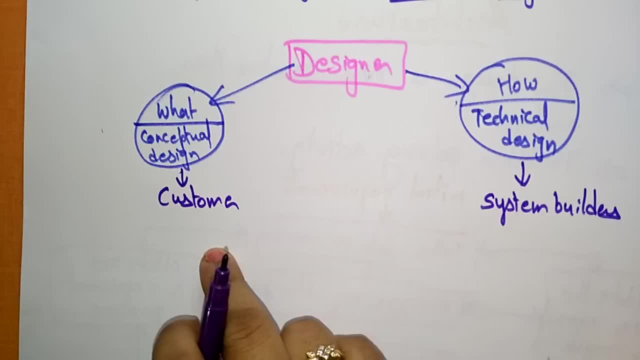 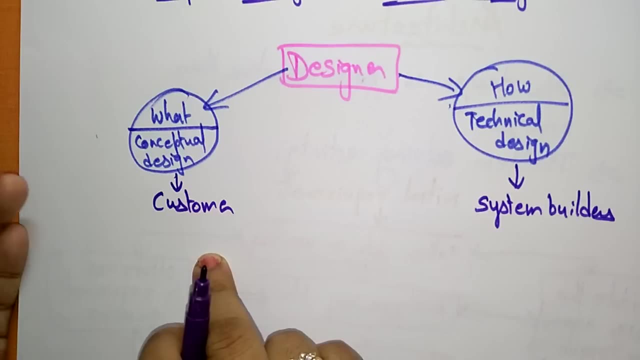 data come from. what will happen to data in system? so, whatever the data that we are putting uh, we are giving. so then, what will happen to data in system and how will system looks to the users: is uh, is it a user friendly or not? so they think about various uh questions. they will be arises. 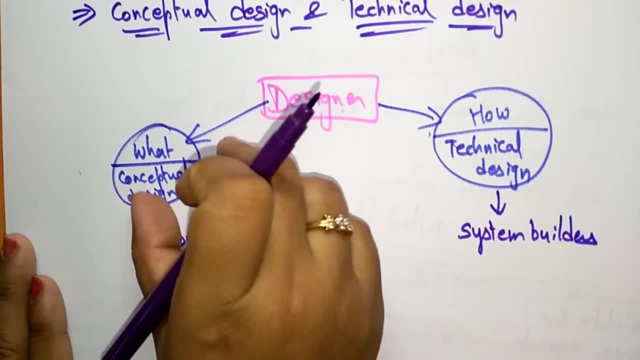 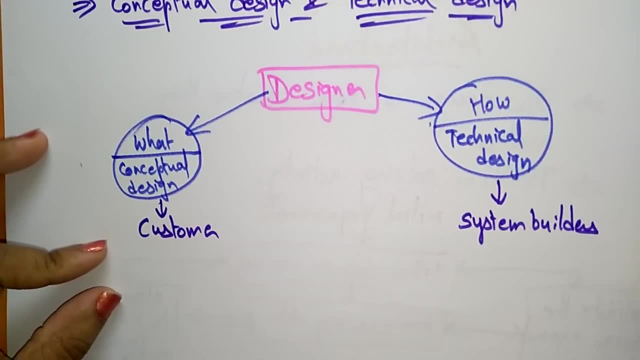 they'll get the answers. with the help of this designer, with the help of the conceptual designer, they will get the answers for all these questions. where will be the data come from? okay, by seeing the design conceptual designer, the customer will understand where will the data come from and 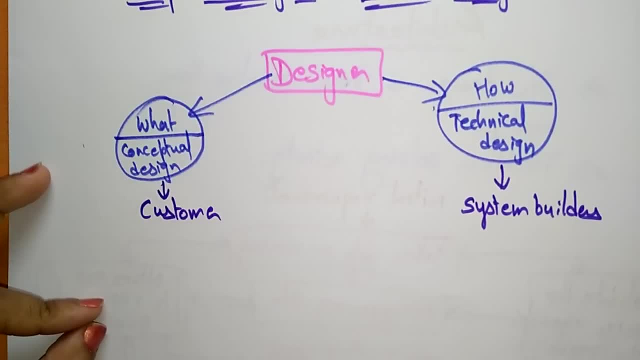 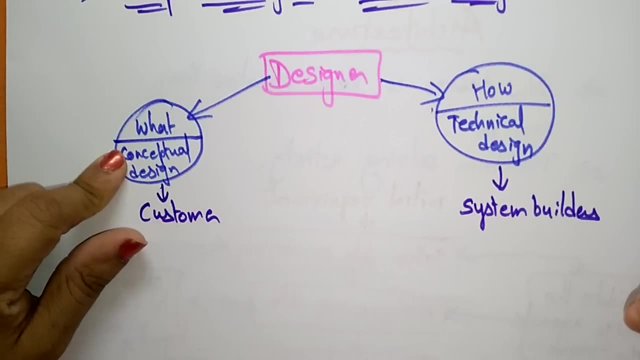 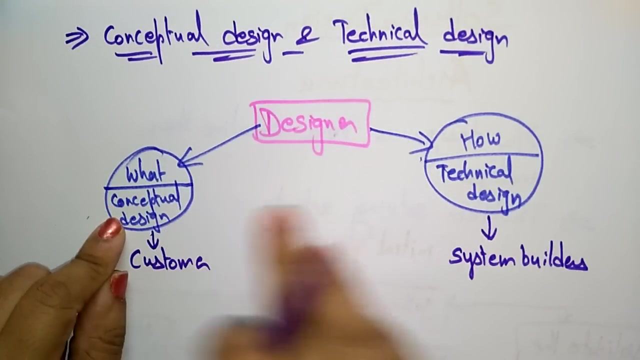 what will happen to the data and system? how will system look to the users? what choices will be offered to the users? everything will be clear to the customer with the help of the conceptual design. so the designers are trying to draw draw two types of diagrams: conceptual designs and the technical designs. the conceptual designs will 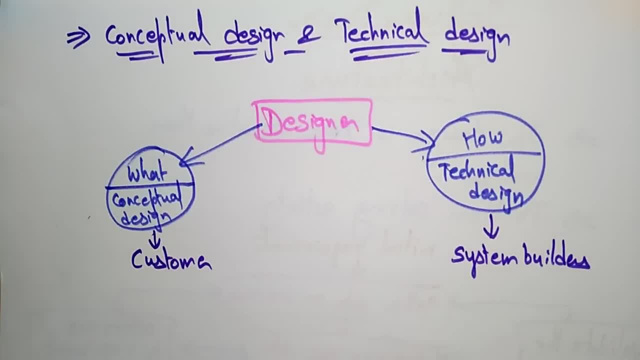 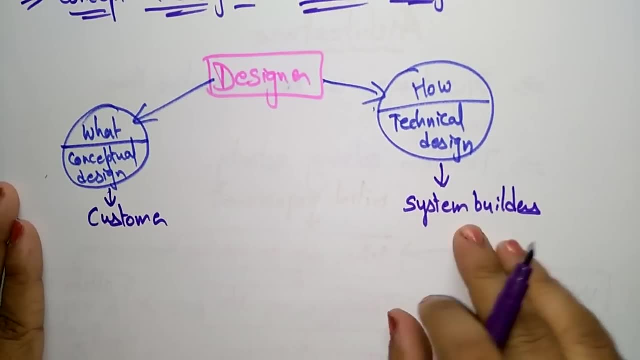 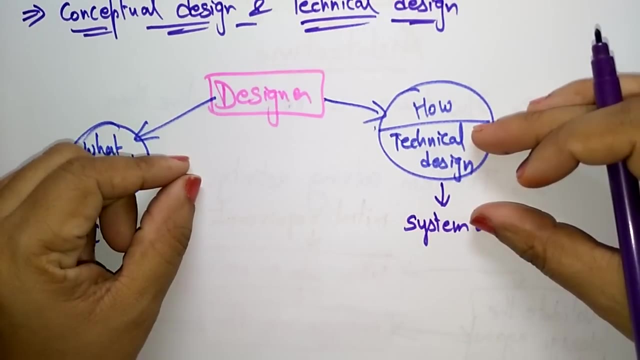 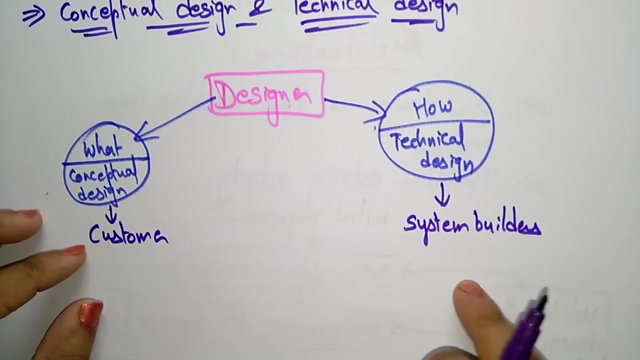 give the answers to the customer queries, whatever the queries they are having. the that will be the answers will be given and coming to the technical designers, so the system builders. so actually what this? how the technical designers will design the product, so they will first describes hardware configuration, software needs. they require communication interfaces, input outputs. 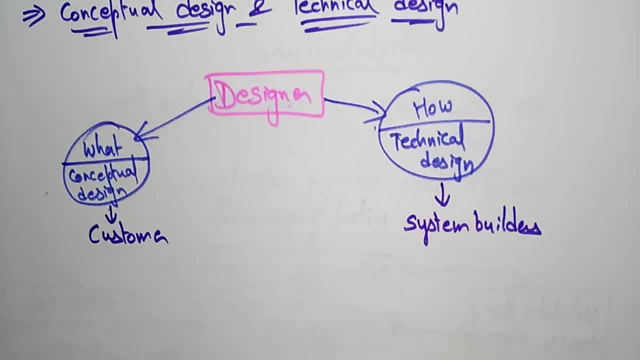 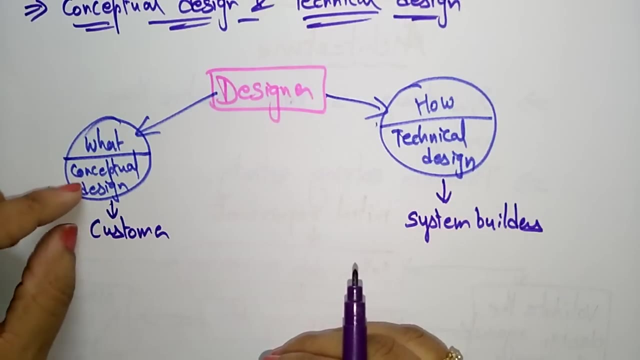 of the systems: software architecture, network architecture, everything will be, they will be designed. so with the help of that technical designs, they can understand what they are going to be implemented, so what the customers will be think. that will be represented clearly in the form of conceptual design so that the customer will get the answers for their queries with the 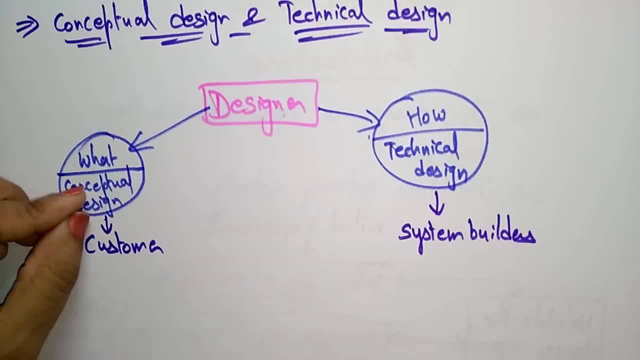 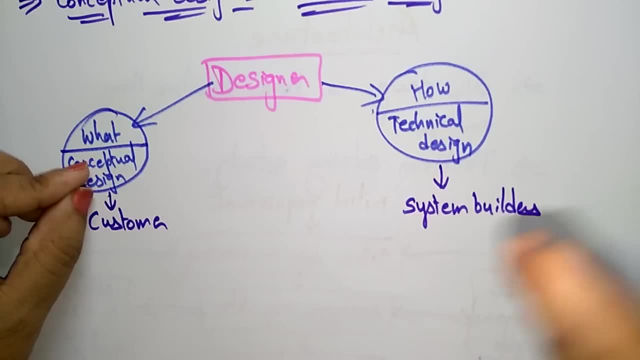 help of the software design, so that the customer will get the answers for their queries, so that the conceptual designs, the technical designers, will always describes about the project. they are going to be implemented in the form of hardware configuration, software needs, communication interfaces, software architecture, network architecture, everything. so this is a two.